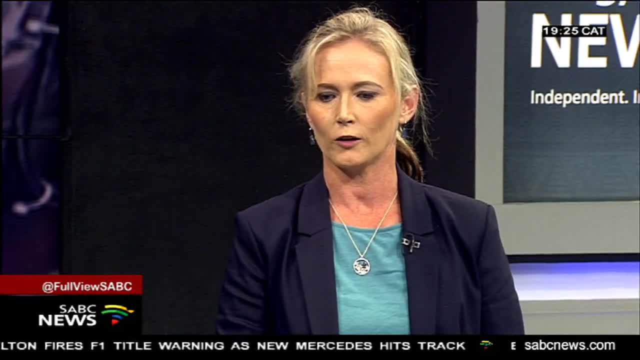 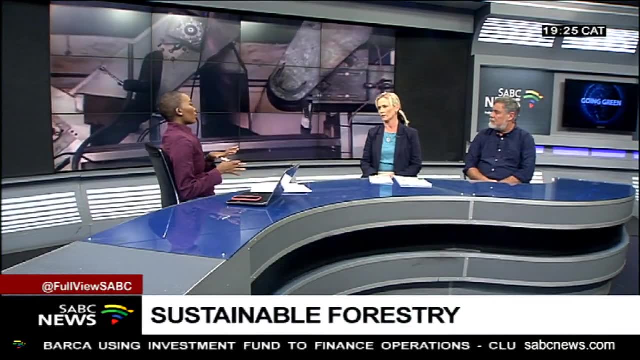 So the forestry sector? actually, while they are harvesting continually and annually, every year, they are also planting trees, the same after they've harvested them on those tracts of land. What's that process like of getting rid of the forest and then building the new ones, and how long does that take? 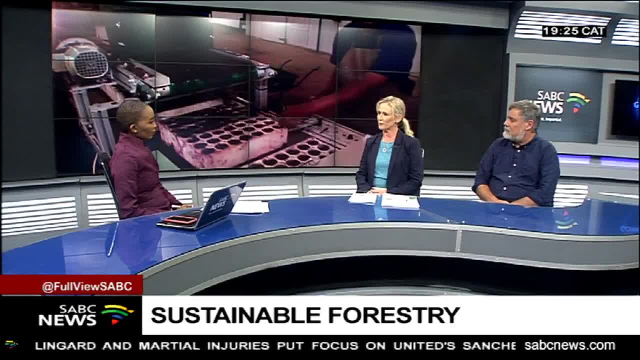 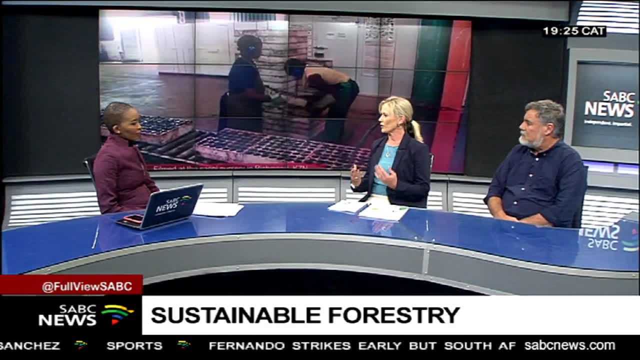 Well, a pine plantation or eucalyptus plantation- and the Prof can probably correct me- but it's about seven to ten years rotation. So it's pretty much like farming- any sort of farming practice, Except your rotations are a lot longer. 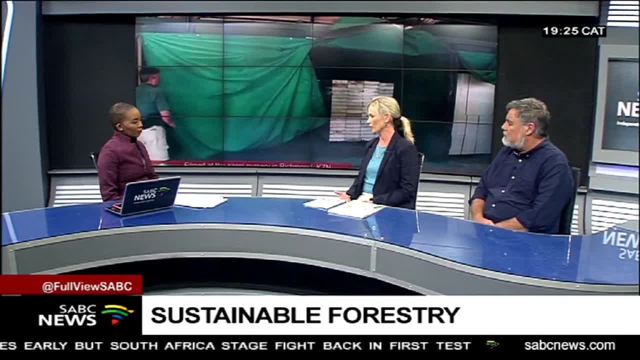 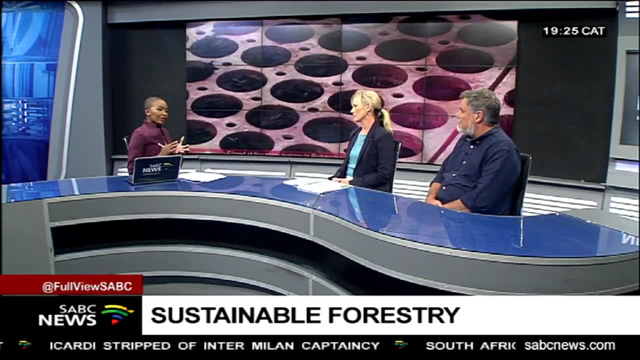 You know, you're harvesting wheat annually or corn annually, whereas with trees you're harvesting them after seven to ten years, depending on what they're used for. And what sort of effect does that have on the South African environment, on the environment around and also the people who may be living close by? 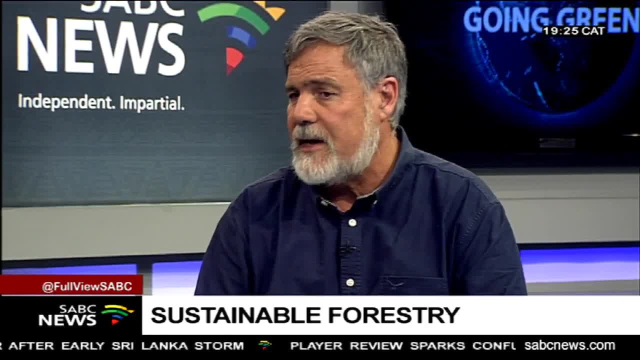 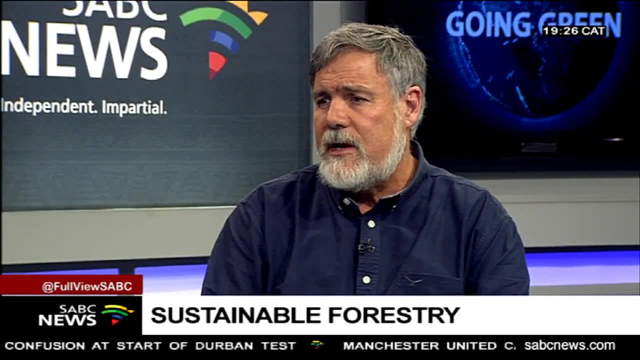 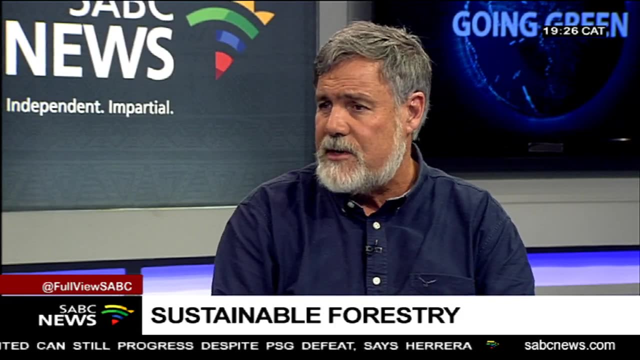 So if we're going to confine ourselves to South Africa, the impacts are largely twofold. The first is that when we plant evergreen, fast-growing trees into former grasslands, the amount of water which appears in the rivers decreases substantially. 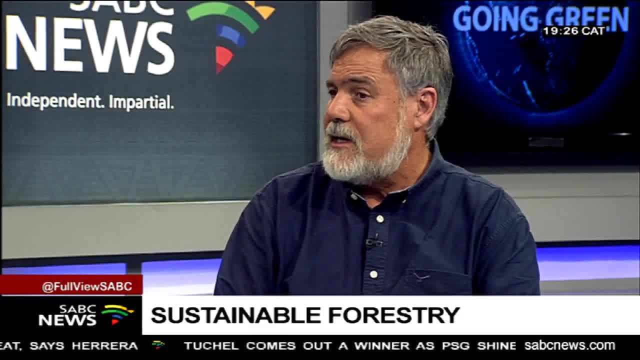 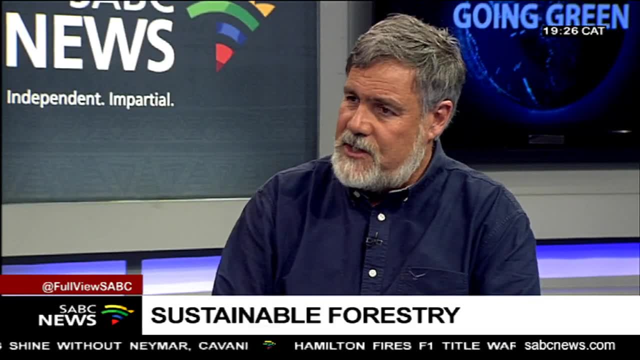 And that was a big surprise to everyone around the world, and South Africa was the leader in research on that topic, And we now know that to be the fact and that's why we do not permit plantations to exceed a certain fraction of the landscape. 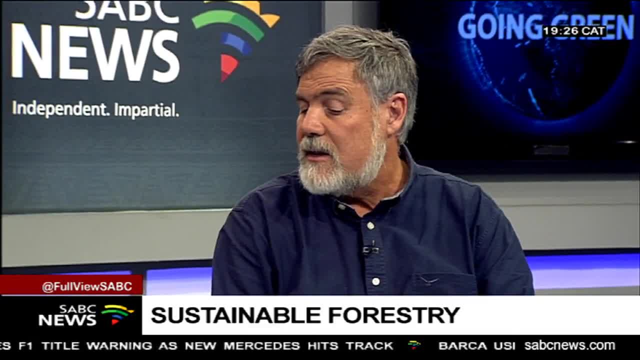 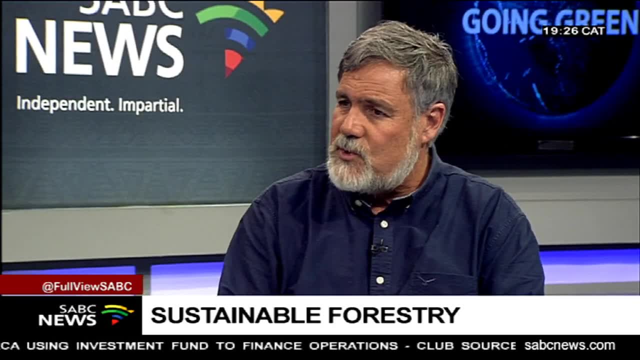 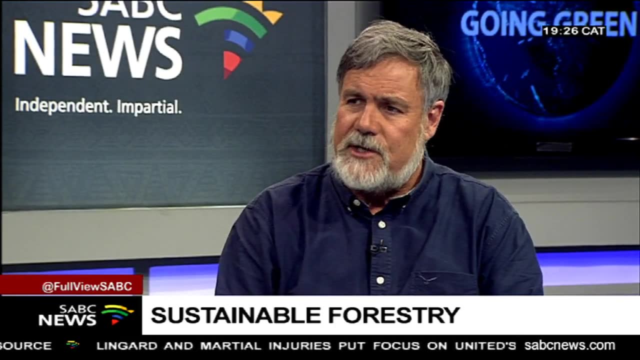 otherwise there isn't water available for other uses. The other major impact is that sometimes the plantations occur into grasslands which were extremely rich in species, and you're replacing that with essentially a monoculture, And so we also have restrictions on where and what fraction of the landscape. 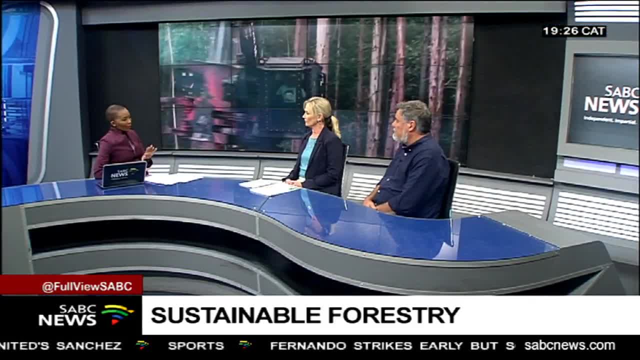 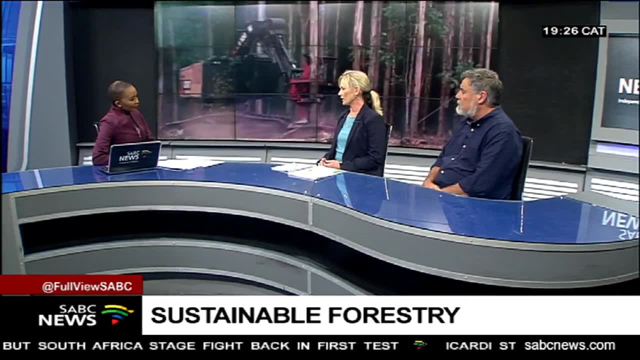 you can plant up in order to protect biodiversity. Let's speak about that word: monoculture. It's come up and there's quite a large criticism of it. What is it and why is that criticism there? So monoculture is really just a portion of land that is dedicated to one single species. 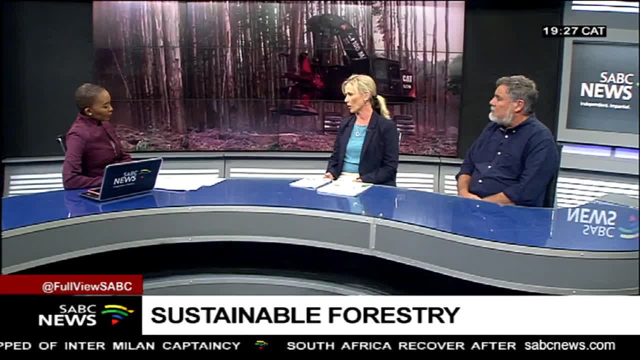 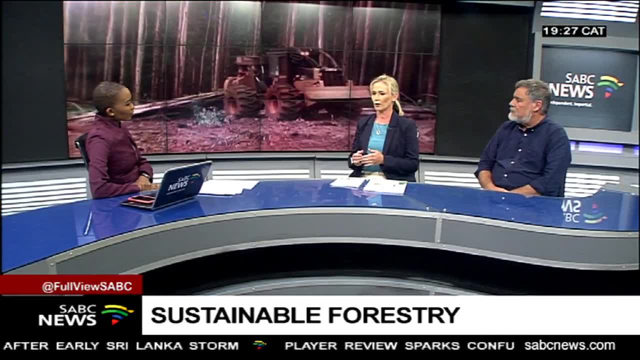 So in the forestry sector it could be pine or eucalyptus and perhaps some wattle, But it's really one species in this one section of land And then obviously in forestry what we're trying to do is try and mitigate those monoculture at landscape level. 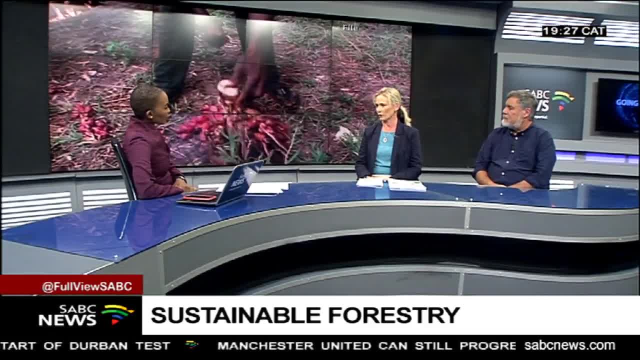 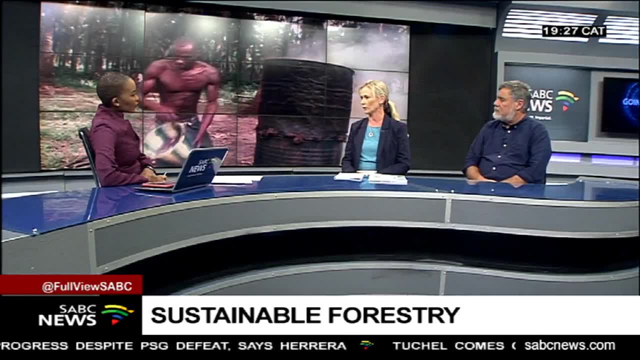 by protecting areas for conservation. So a lot of the areas in the forestry-owned land is reserved for conservation and biodiversity and to mitigate the impacts on biodiversity. So if you go into a planted forest in, say, Pumalanga, you'll also find 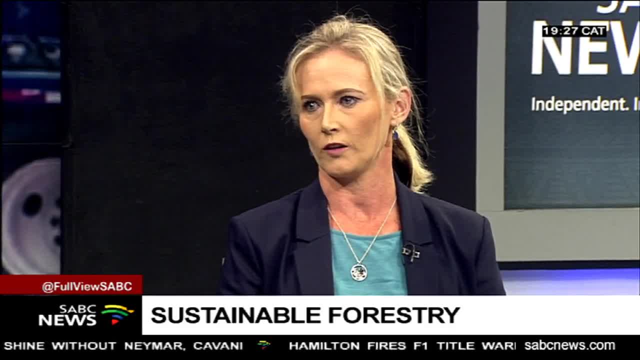 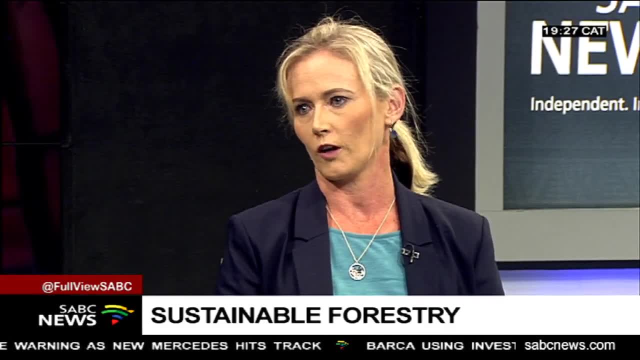 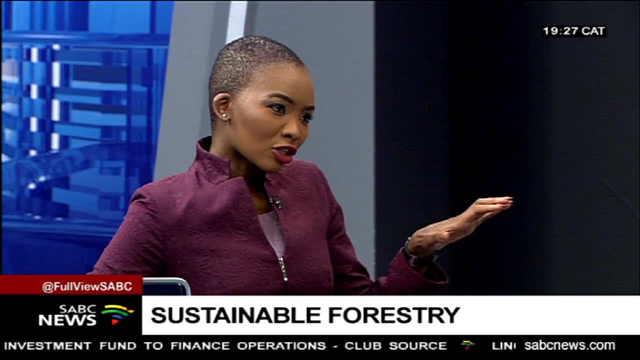 nearby areas of rich, rich biodiversity and a lot of species conservation. There's lots of species that have almost re-occurred in some areas thanks to the efforts of forestry. So what effect does that have? planting one specific thing, I know you've spoken about the biodiversity that's around it. 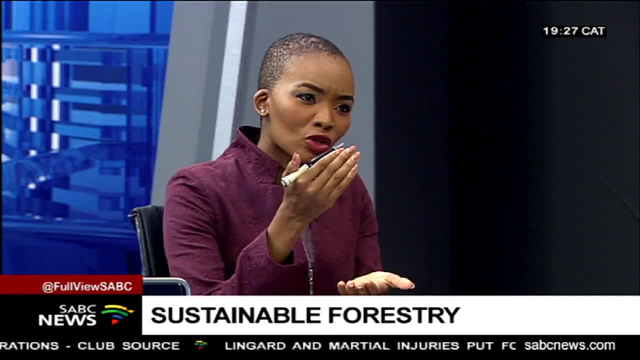 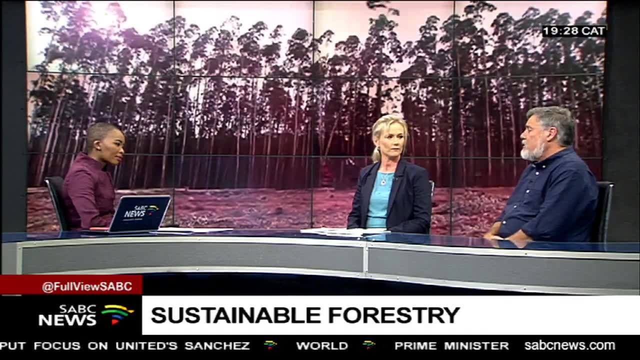 but in that specific section, what happens to that soil? What happens to the ground that those things are planted on? So the answer to that is quite complicated. When you have lots of species in an ecosystem, that ecosystem tends to be a bit more resilient. 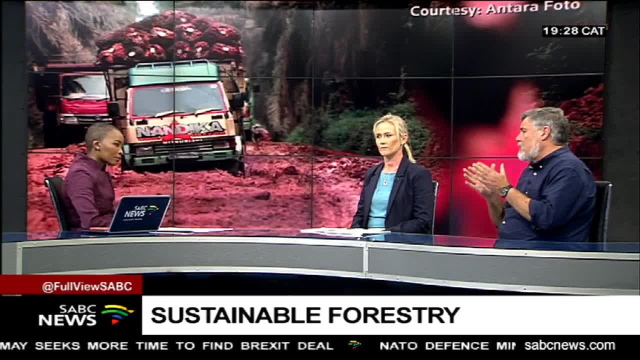 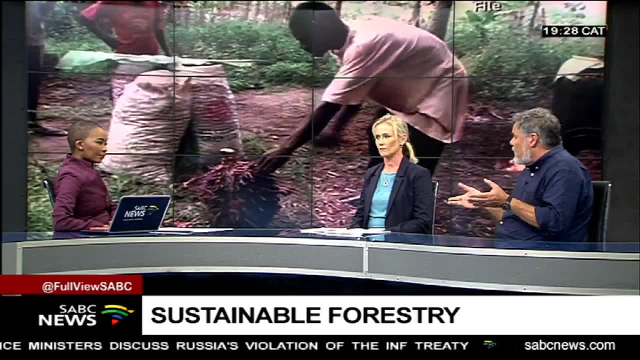 than if you just have a few species. Just imagine, for instance, you've planted a large area to just one thing and a particular pest comes in or a particular sequence of weather that it can't cope with. then you lose all of it. 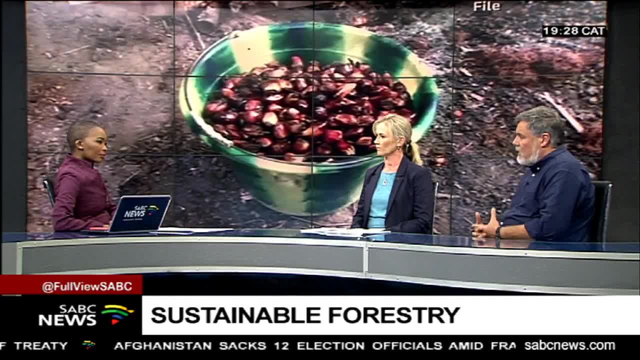 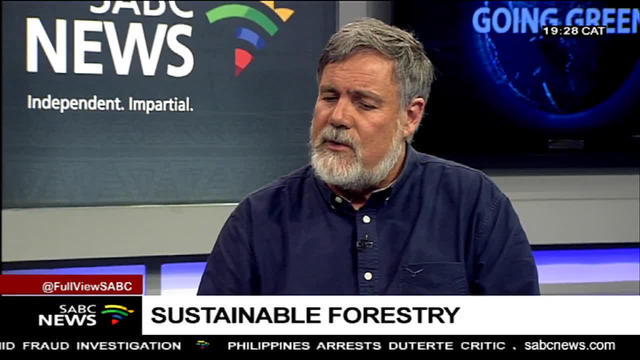 Whereas if you've got lots of species, they can compensate for one another a little bit. So you might ask: well then, why do people only plant one species? It's largely because if you're harvesting out of an ecosystem, usually it's only one or a few species. 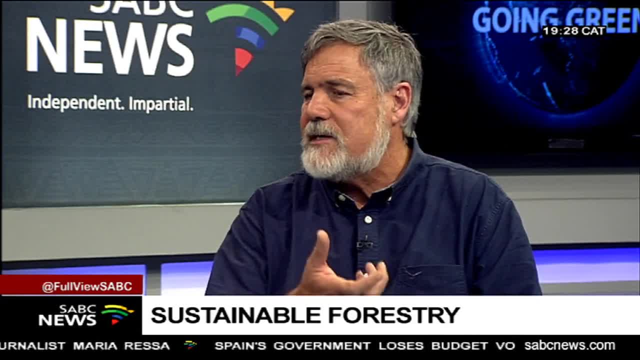 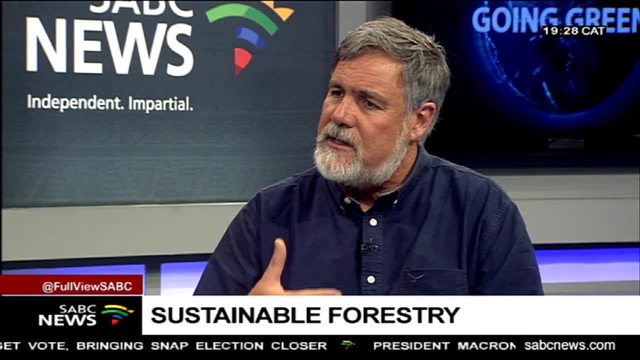 which are providing the value that you're looking for and the rest, in a sense, are taking up space, And how that planting propagates then into diversity in things like in the soil and in the birds and in the insects. there's a sort of a knock-on effect there as well. 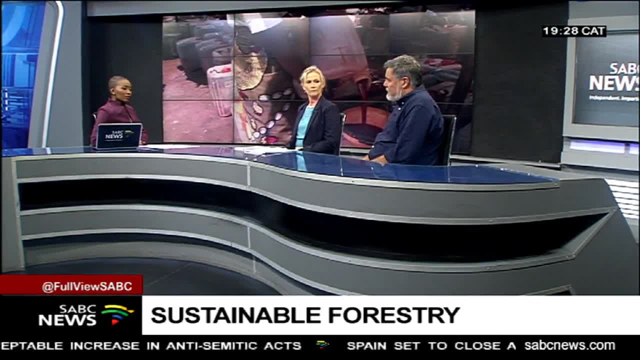 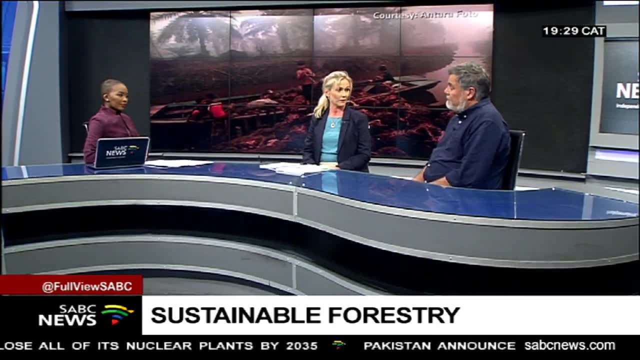 And so you have to follow this all the way through the ecosystem. How would you then characterise the health of South African forests now? Yeah, I think- and Prof can back me up or not- but it's a good, our forestry sector is in a good space. 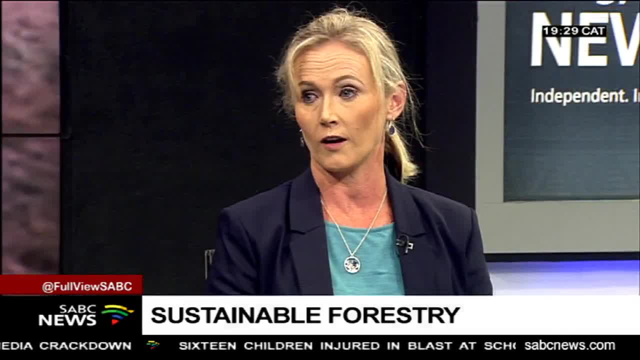 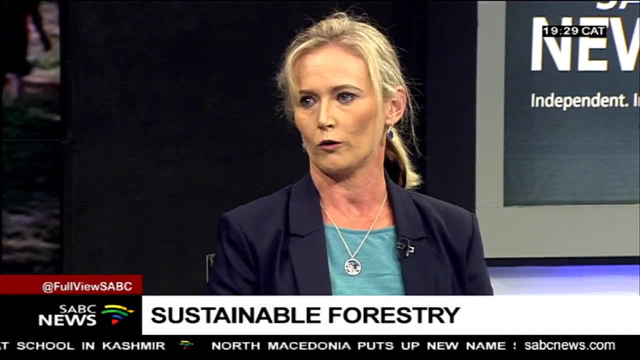 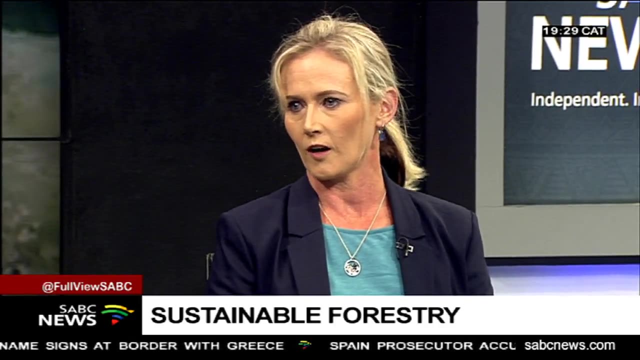 We do have issues around certain pests and diseases which are as a result of climate change and just changes in temperatures in some places. But we're doing a lot of work to try and mitigate that and look at ways to treat these pests and diseases with ecologically sound methods. 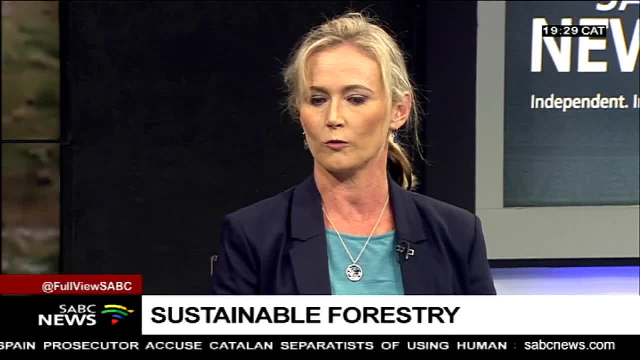 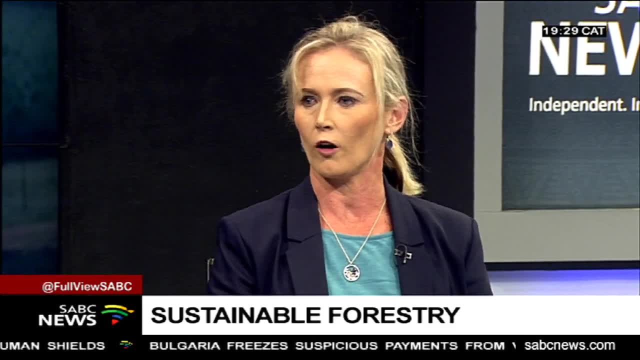 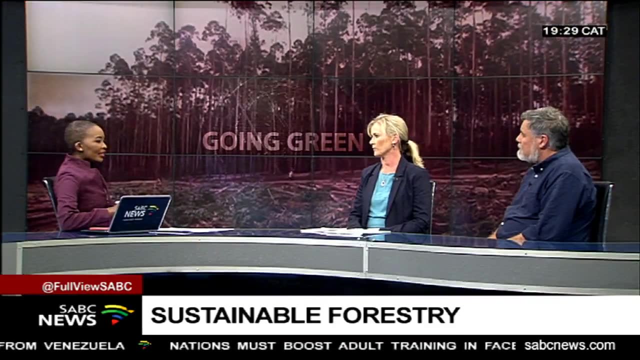 A lot of work going into the pesticide projects and to make sure that things like biological control the Cyrex wasp- there's certain other insects that will prey on that particular wasp- to help mitigate the damage it causes to the trees. When we began, we spoke about the health of Southern Africa. 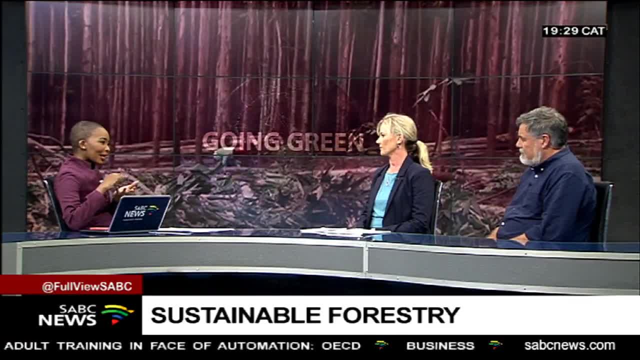 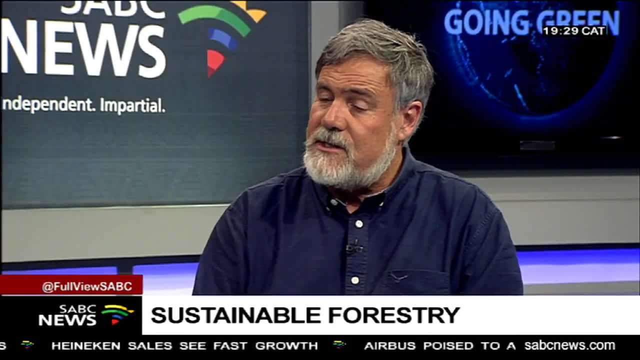 deforestation. Talk to us about that and climate change, how it's affecting the rest of the continent, if South Africa's looking slightly better. So the big deforestation, as I say, is in woodlands, and that's the same around the world. 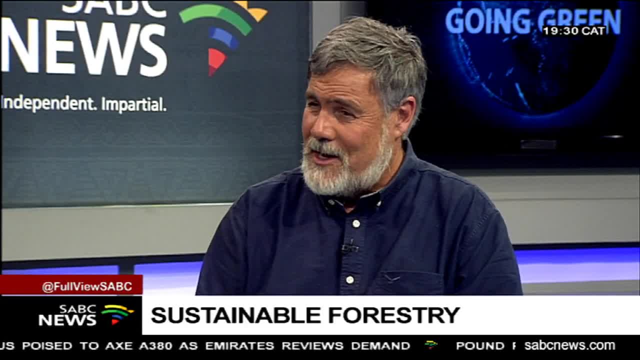 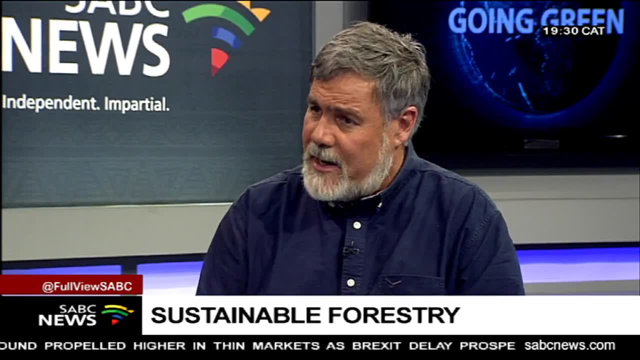 We all hear about the Amazon deforestation. I've lived and worked in the Amazon. It's still there because the tropical rainforests are a horrible place to live in and do agriculture. They're too wet and the soils aren't good. 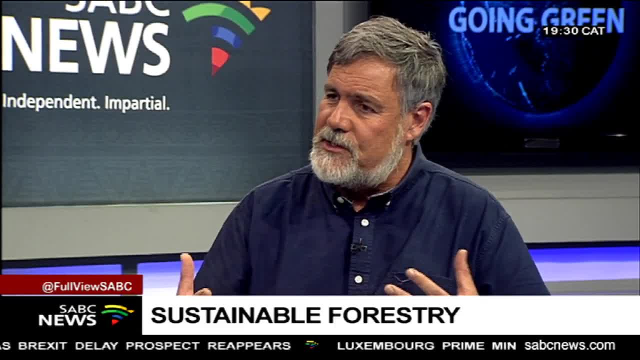 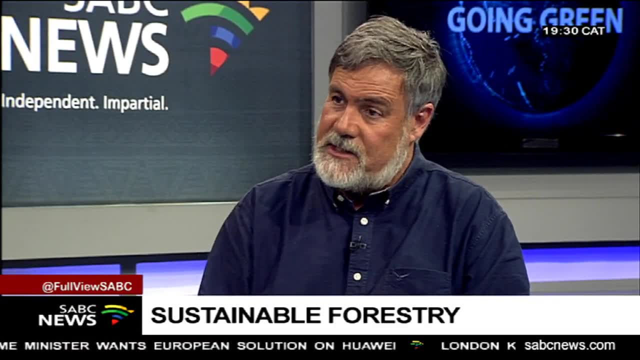 So where the deforestation occurs is on the fringes, in these drier forest types, woodland types which are on deep, well-drained soils, And that's what's happening in Southern Africa, And that's being converted largely into large crops of mud. 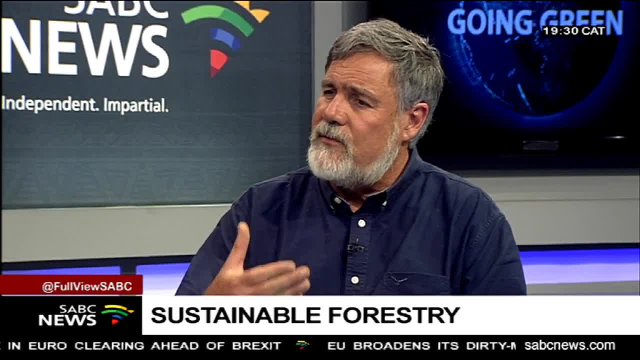 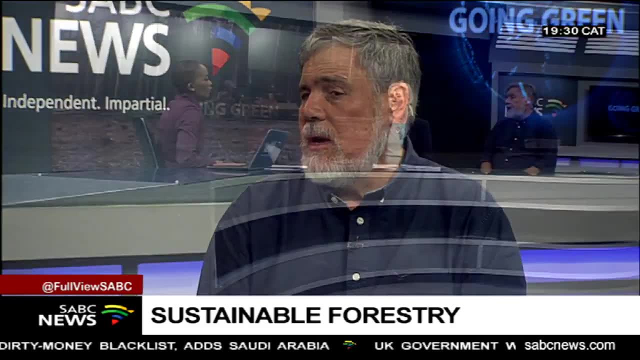 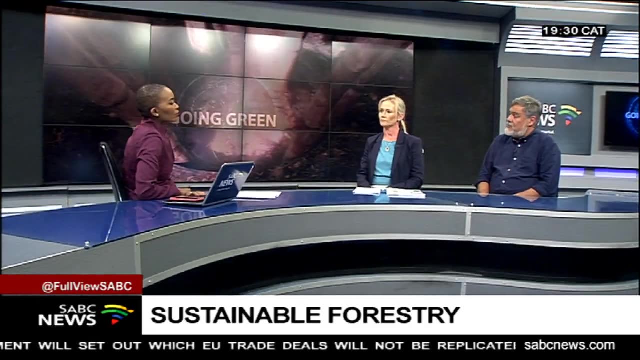 Maze and soybean Not to supply food in Africa mostly. It's mostly commodity exports being driven by dietary changes around the world And that has negative impacts on our biodiversity. It's worrisome in the sense that all Africa's major rivers 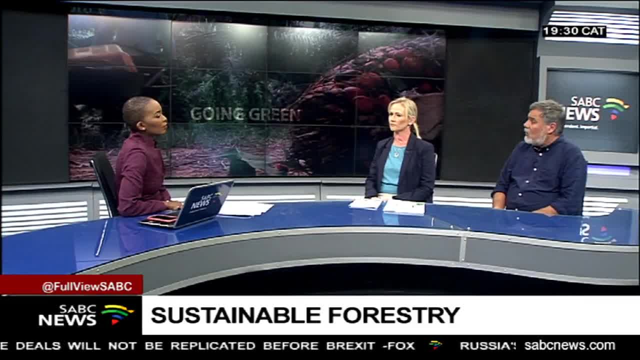 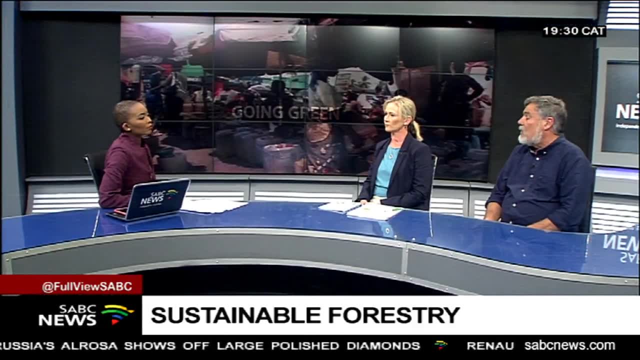 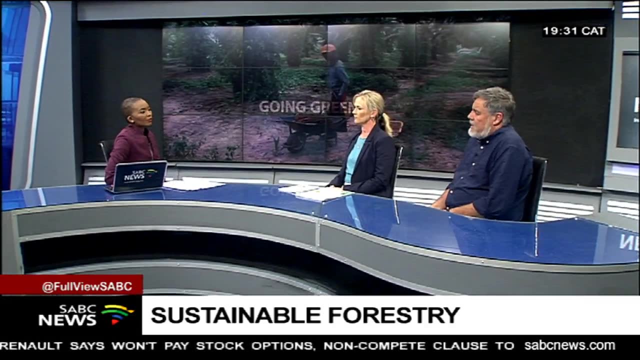 especially those that flow in the Southern African area, all have their origins there. So the Zambezi and the Kavango and the Ruaha all rise here. So there's a threat to that water resource And there is a net movement of carbon dioxide. 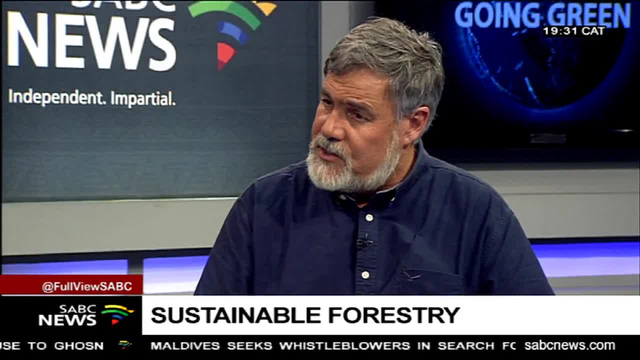 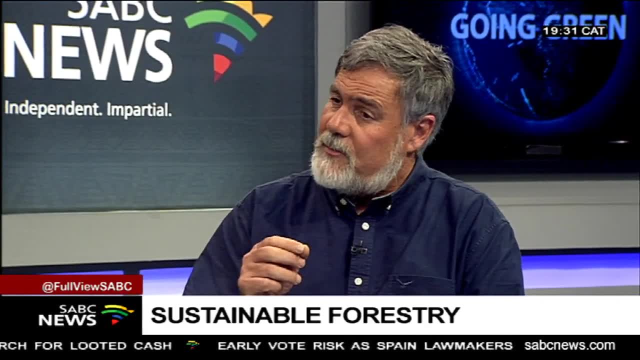 from being held in the bodies of those plants and in the soil underneath them, especially into the atmosphere. when you convert the forest into agricultural lands, When you add that up of an area as large as the belt that's affected, it can make quite a significant difference. 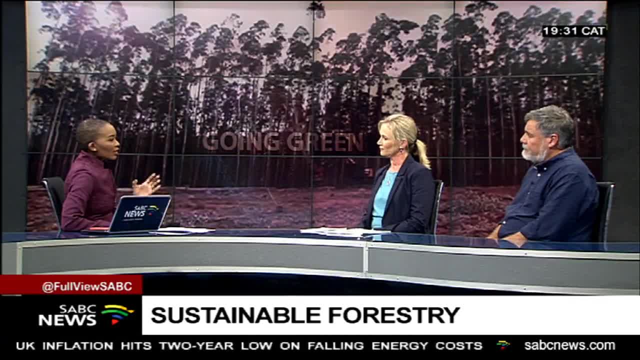 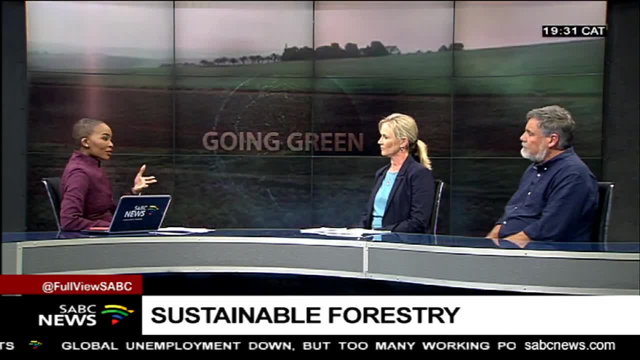 to the global climate, Mm-hmm. Earlier on we spoke about the effects that monoculture specifically can have on rivers. the unexpected effect. We know that South Africa is a water-scarce country. We had that big drought scare. well, the big drought in Cape Town. 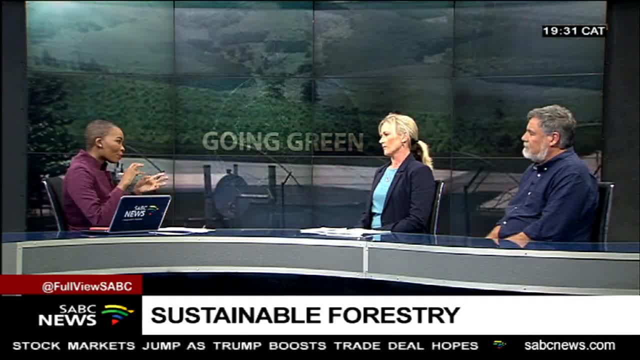 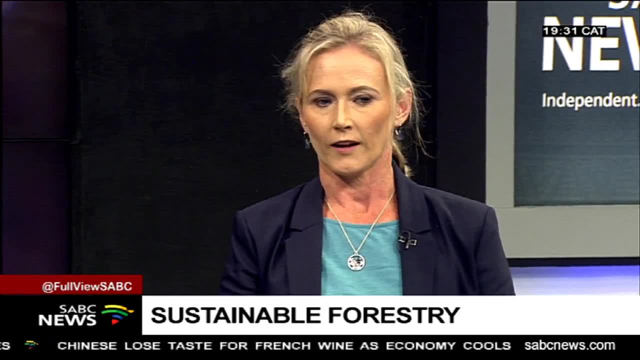 How do you then mitigate this And what's the state of our rivers at the moment, And how do you balance this? in forestry as well, There's a lot of work being done to remove alien and invasive species. So in Cape Town there's been a lot of work to remove pine species. 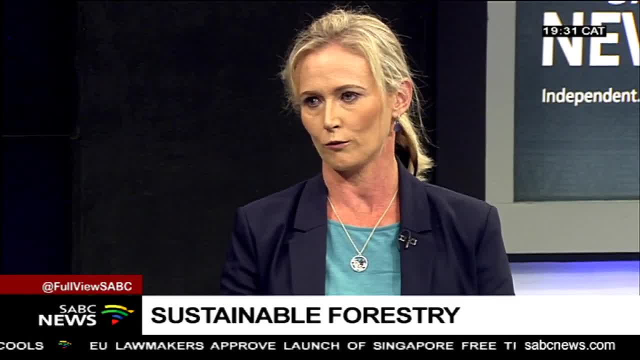 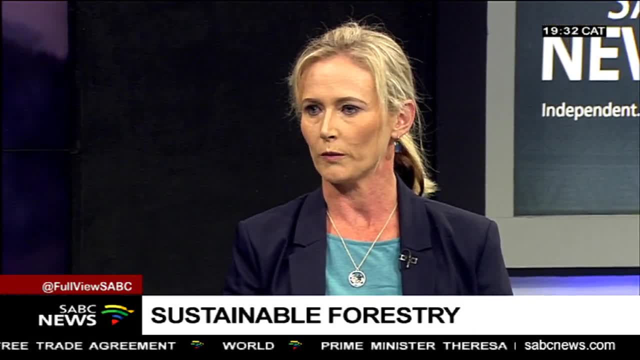 and eucalyptus trees where they may have sprouted in the sort of riverine areas. I can't personally speak on the actual water health, but there's also a lot of work being done on the wetlands to remove trees and have a buffer zone between the rivers. 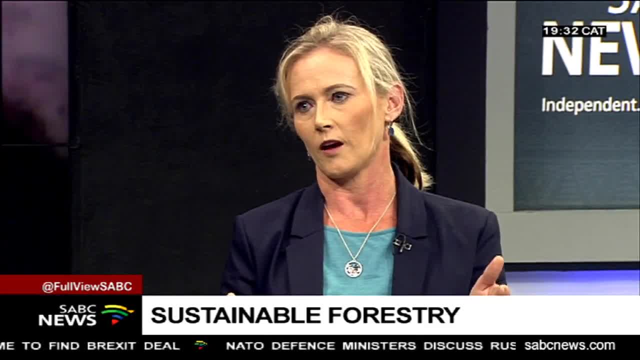 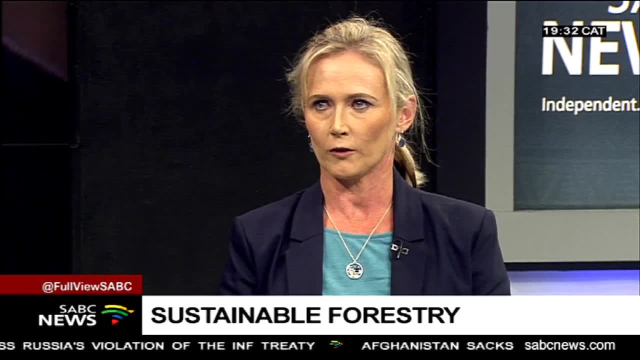 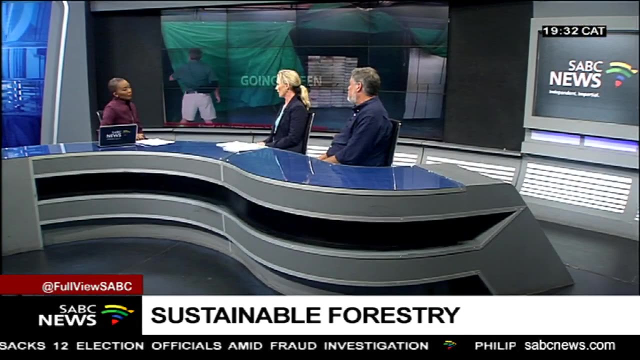 and between the plantations and the rivers to ensure that we don't impact on the streamflow any more than we do in forestry- And we know forestry is a streamflow reduction activity- and they are not irrigated. Plantations are not irrigated much like other agricultural crops. 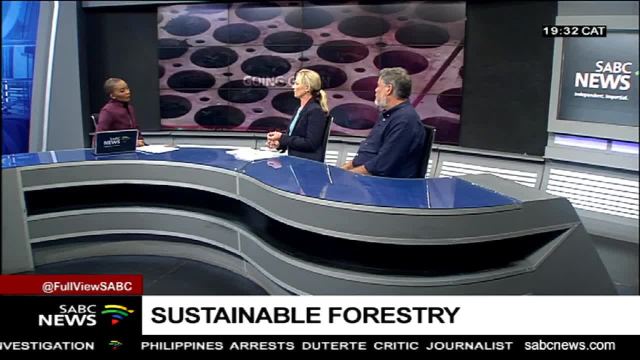 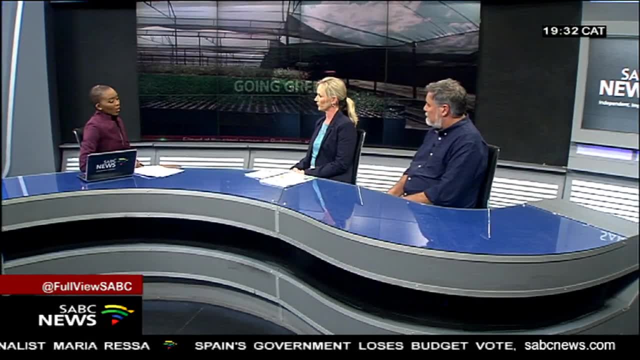 And so we get our water from the rain, but that rain then gets captured by the trees and gets soaked up by the roots of the trees and then reduces what goes into the rivers, as Prof alluded to earlier, When we're speaking about climate change and deforestation. 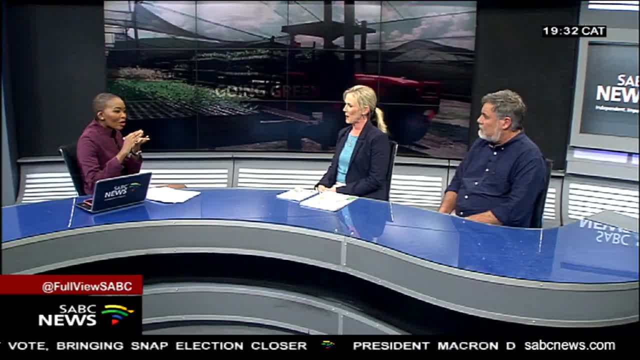 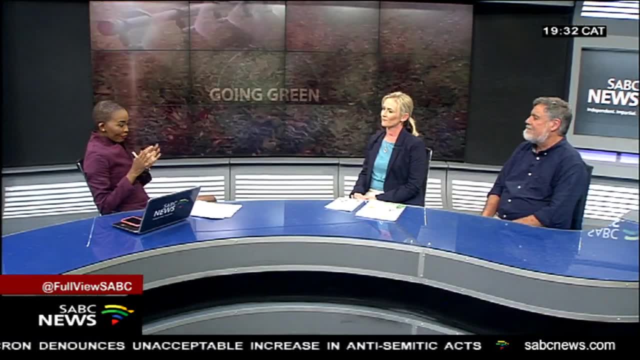 I've heard that that number's, 1.5 degrees, is the safe amount, the safe temperature that we can rise every year. if we're not going to have complete care when it comes to climate change, Are we doing enough, specifically in a South African context? 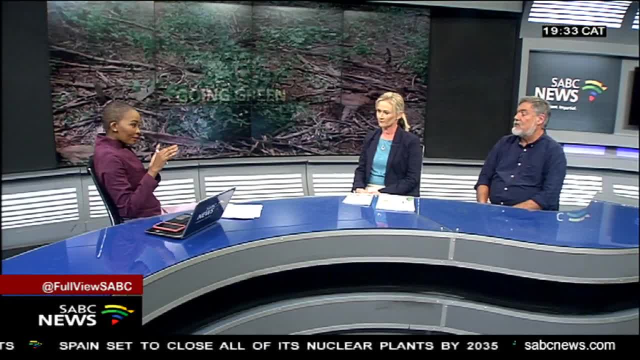 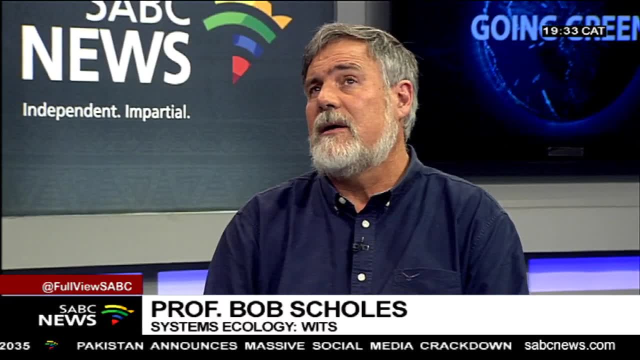 to try and make sure that we're playing our part to make sure it doesn't go above that. So it's 1.5 degrees forever, not per year, And we're well over one already this year. So there's a very small margin of safety. 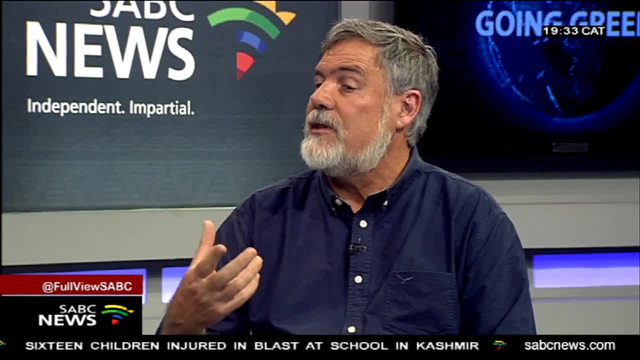 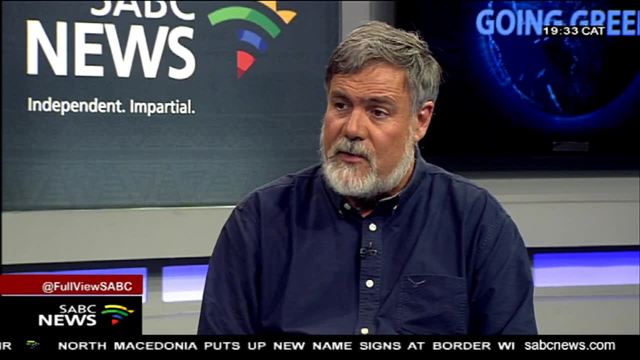 and basically the world has to turn the corner within the next 12 years if it's going to stay below 1.5 degrees Celsius. South Africa's contribution to that is very, very small. It's about 1% of the global forcing on the climate. 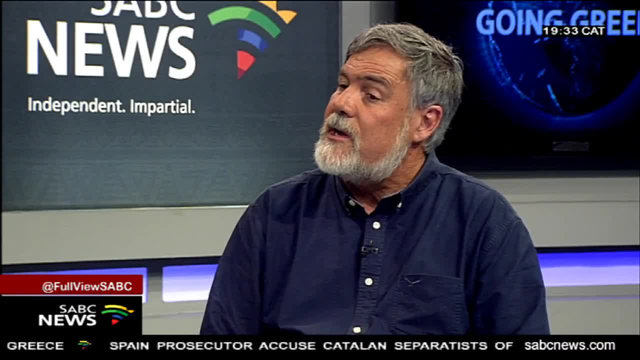 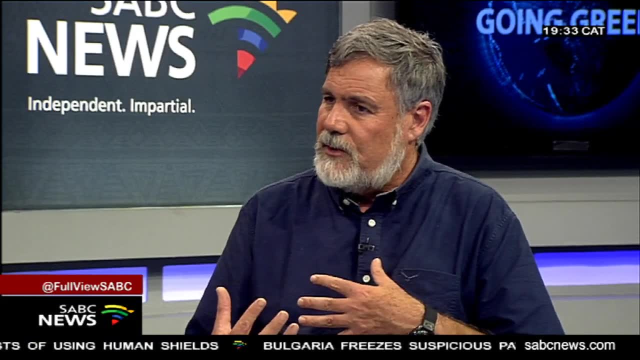 But we're extremely affected by climate change. Our climate is already warmed up by more than 1.5.. We're already warmed up by 2 degrees. We amplify climate change here, So we're very vulnerable, but there's not that much that we can personally do about it. 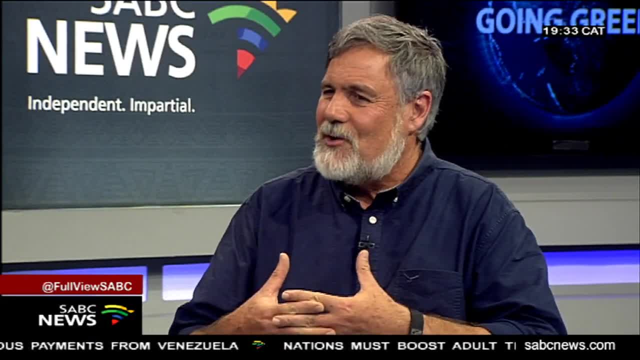 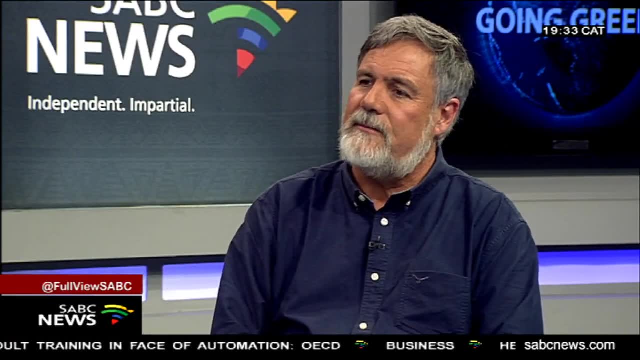 And that means that we have to focus our energy on moral suasion of persuading the rest of the world. guys, this is a really bad idea. let's all get together and do something about it. I know you said there's not much you can do. 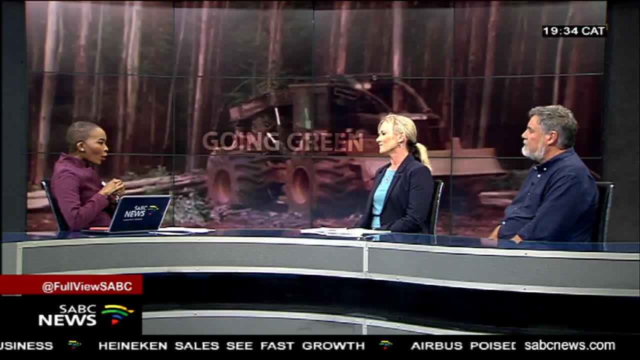 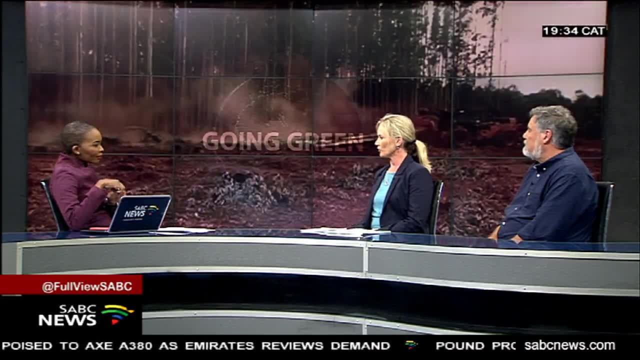 but when you're reading up on climate change, people are saying: you must make sure that you're using recycled boxes. When it comes to paper, there's specific paper you can use. Well, I think, as consumers, you just need to be responsible. 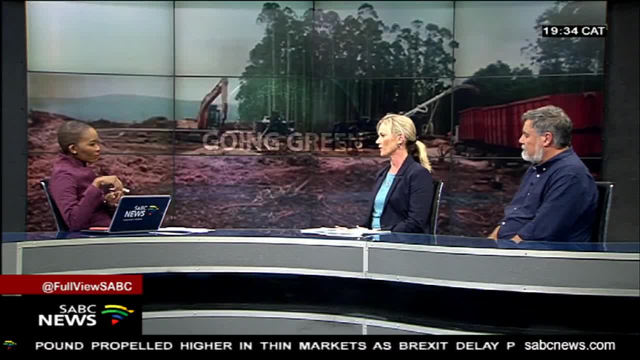 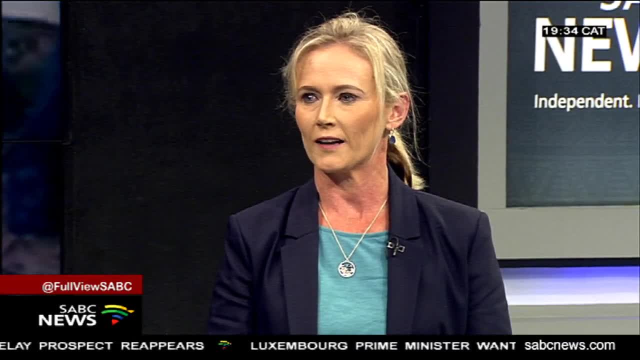 about where you source your paper. Look for symbols such as the Forestry Stewardship Council mark, the FSC mark, PEFC, and look for products that are sustainably sourced, Recycling your boxes while it doesn't save trees, because trees are farmed to produce paper. 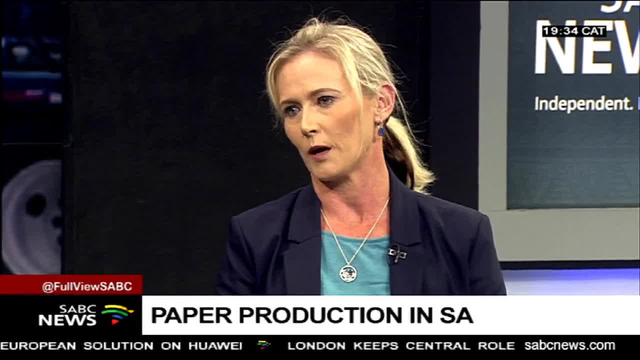 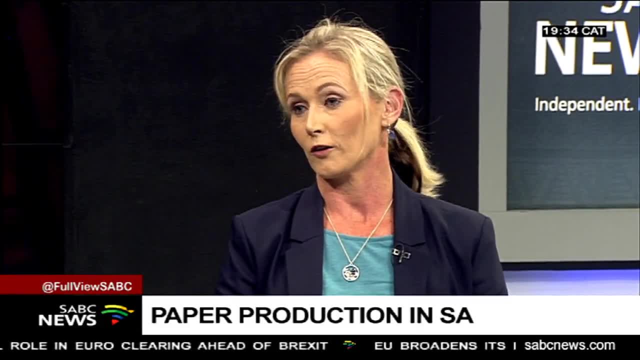 it does keep that carbon that's absorbed by the tree locked up in the paper for longer. So there are little ways that, as citizens, we can help mitigate our impact on the environment. And if we look at the African continent as a whole, would that change at all? 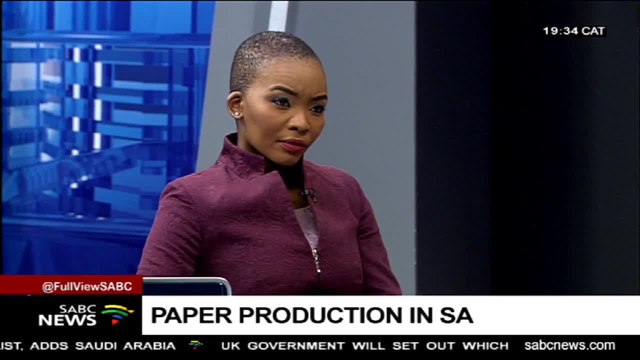 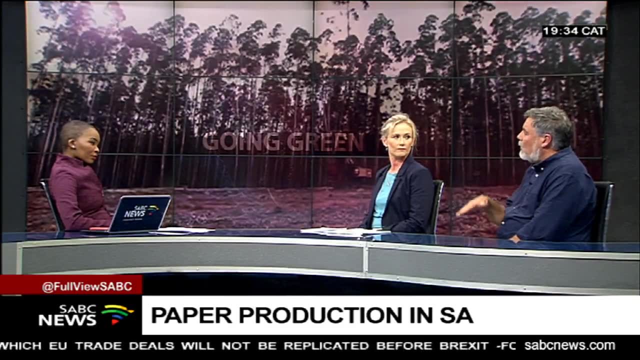 Would that answer be different? Yes, I think it would. The big choice for the African continent is: do we go down into this sort of deep hole of degradation and then claw our way up the far side? And that may or may not be possible. 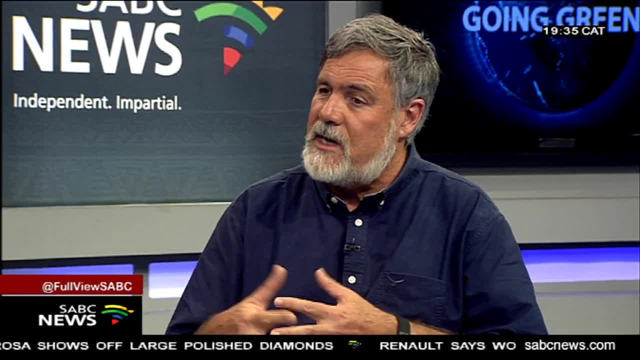 given the state of the world by that stage, Or do we step across it? Do we learn from what's happened elsewhere and say no, there's in fact a different development path. We, for instance, don't need to convert those woodlands. 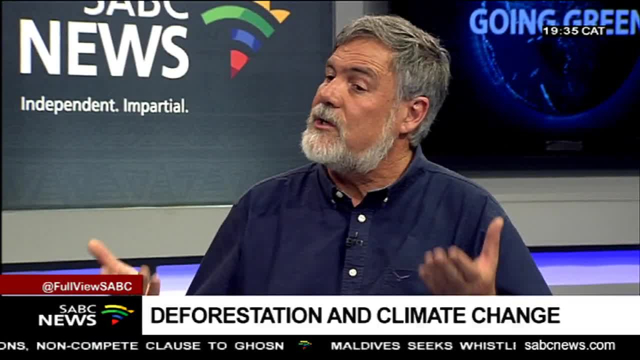 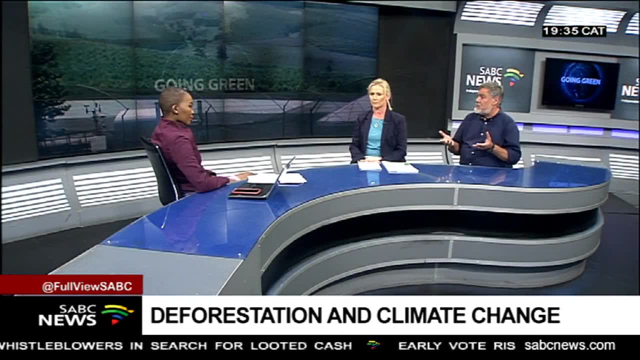 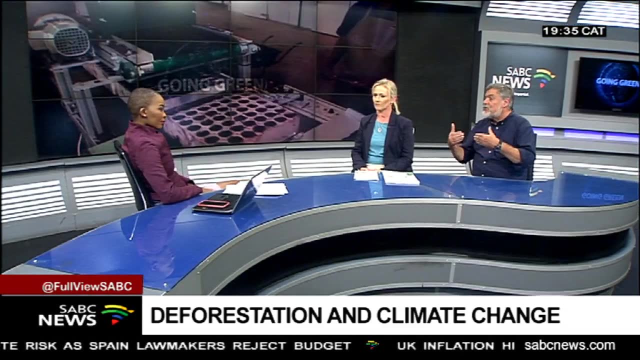 into endless maize and soybean fields. We could turn them into agroforestry, which is higher value, more diverse and better for that landscape. So we have choices which face us. We don't have to go the industrialization path which other continents have gone, just because they went there. 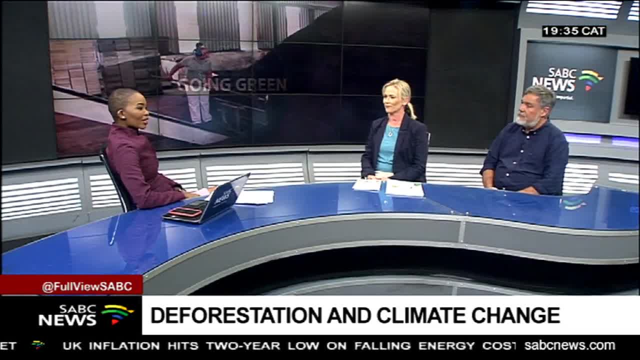 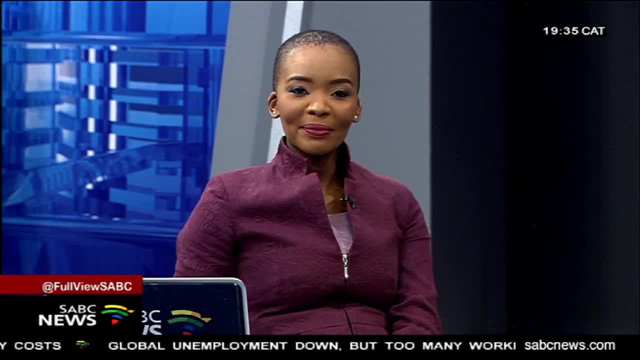 We can be smart about this. Thanks both so much for your time, Professor Bob Scholes from the Department of Systems Ecology at WITS and Samantha Choles from Forestry SA and PAMSA.